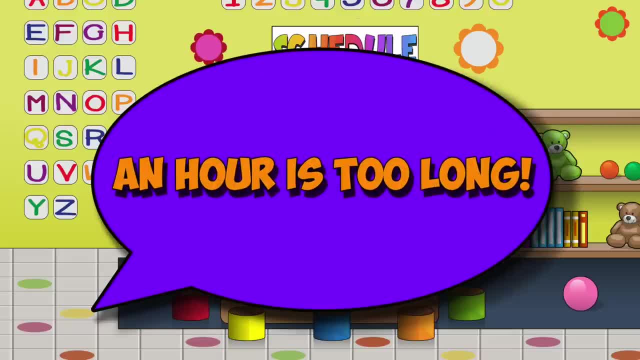 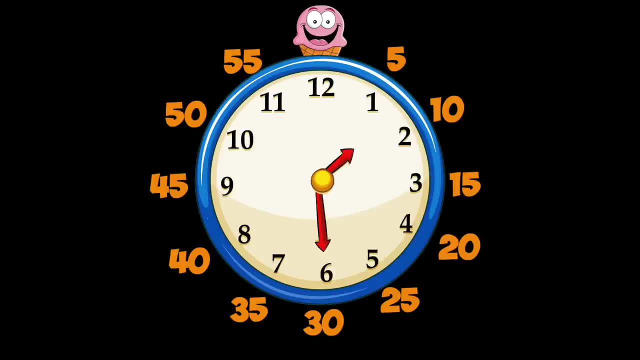 But every student wanted to sing. An hour is too long. It was 5,, 10,, 15,, 20,, 25,, 30.. That's a half hour and we're still really hungry. 35,, 40,, 45,, 50,, 55,, 60.. Where's our ice cream? Well, 60 minutes is. 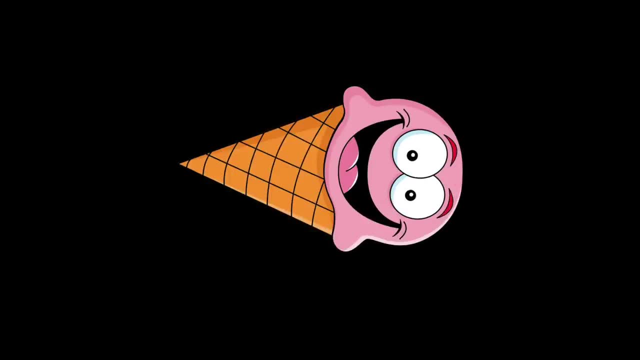 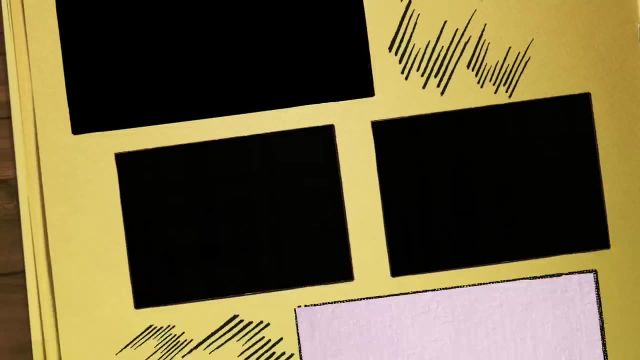 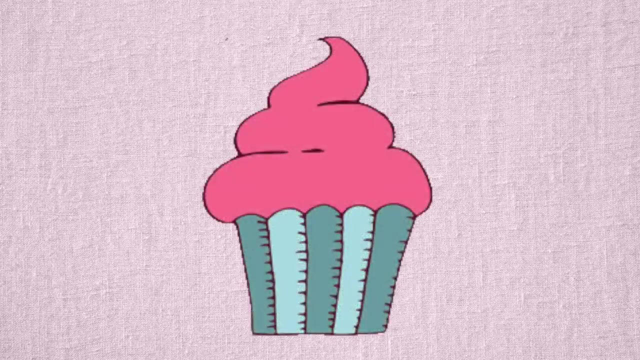 one hour. so I guess it's ice cream time. And then came Tuesday. Our class came in from recess and we had run around. Now we were starving really bad. Our tummies made this sound. Our teacher said there's cupcakes. We would have to wait Exactly for one hour. 60 minutes was our. 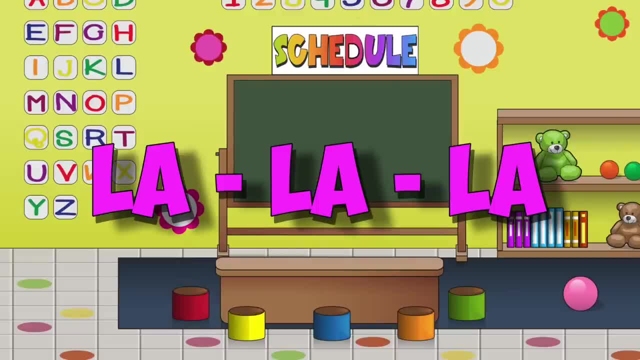 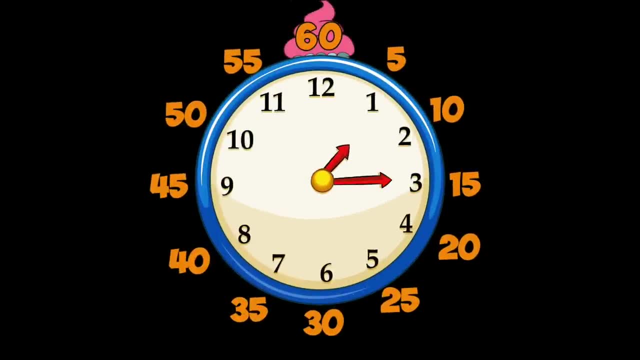 fate. Our teacher started singing a 60 minute song, But every student wanted to sing. An hour is too long. It was 5, 10,, 15,, 20,, 25,, 30. That's a half hour and we're still really hungry. 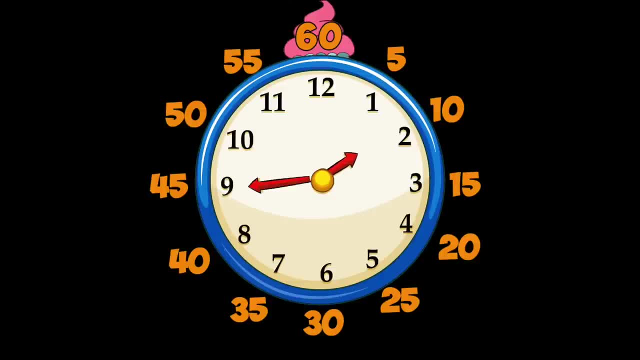 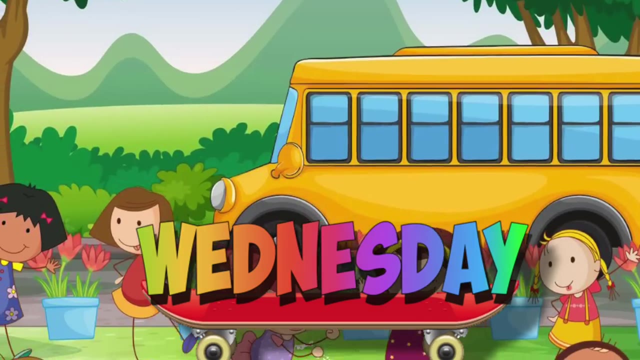 35,, 40,, 45,, 50,, 55,, 60. Where's our cupcakes? Well, 60 minutes is one hour, so I guess it's cupcake time. And then came Wednesday. Our class came in from recess and we had run around. Now we 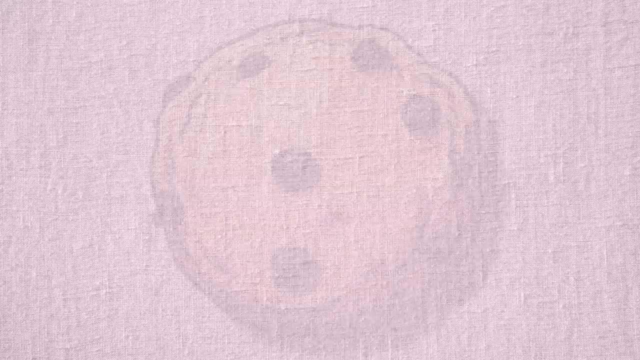 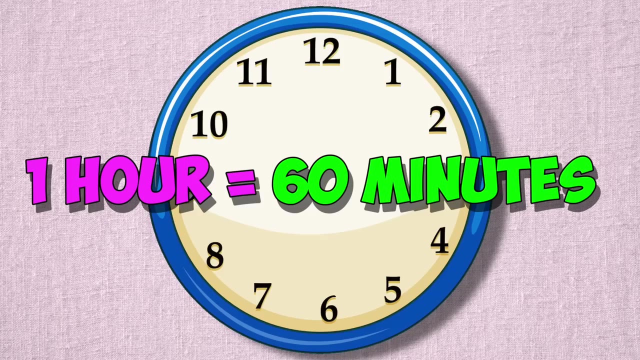 were starving really bad. Our tummies made this sound. Our teacher said there's cookies, But we would have to wait Exactly for one hour 60 minutes was our fate. Our teacher said there's cupcakes. We would have to wait Exactly for one hour 60 minutes was our fate. Our. 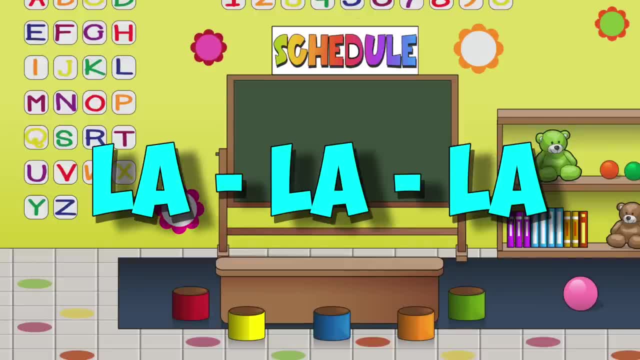 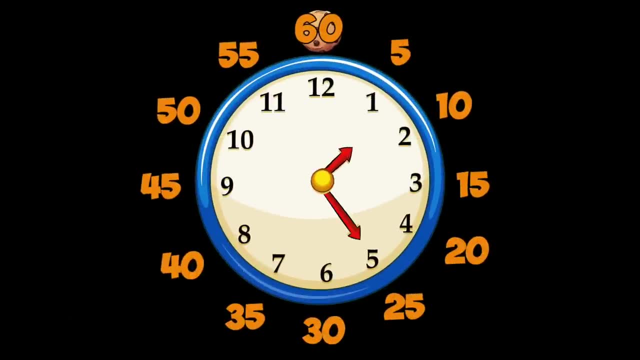 teacher started singing a 60 minute song, But every student wanted to sing. An hour is too long. It was 5, 10,, 15,, 20,, 25,, 30. That's a half hour and we're still really hungry. 35,, 40,, 45,, 50,, 55,, 60. Where's? 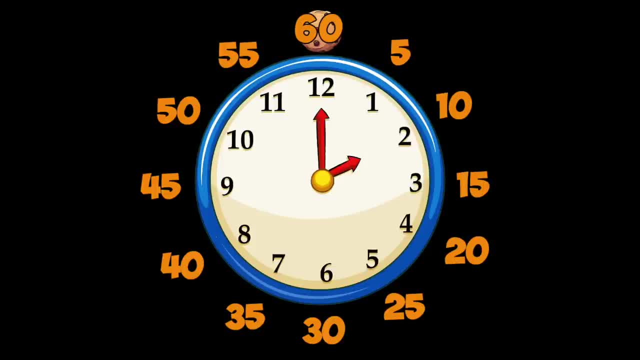 our cupcakes. Well, 60 minutes is one hour, so I guess it's cupcake time. And then came Tuesday, Our class came in from recess and we had run around. Well, 60 minutes is one hour, so I guess it's. cupcake time. But every student wanted to sing. An hour is too long. It was 5, 10,, 50,, 50,, 60. That's a half hour and we're still really hungry. But every student wanted to sing. An hour is too long. It was 5,, 10,, 50,, 50,, 50,, 30. That's a half hour and we're still really hungry. 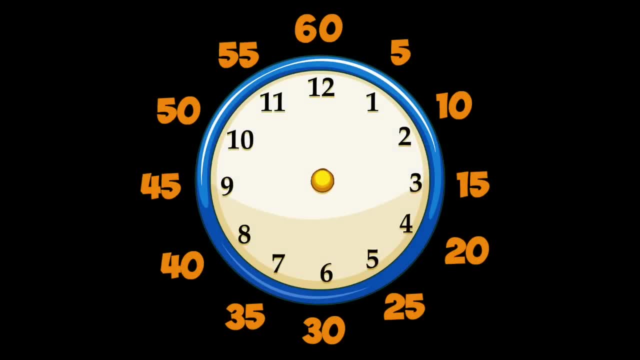 Now let's review. The long hand on a clock shows the minutes and the small hand shows the hour. We always say the hour or where the small hand is pointing first. For example, this clock shows 3 o'clock because the small hand is pointing to the 3. 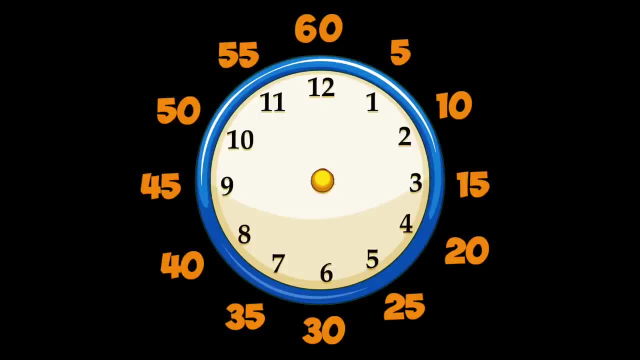 and the long hand is pointing to the 12. If we want to show 3.15,, we start with 3 o'clock and then we can count by 5's until we get to 15.. 5,, 10,, 15.. 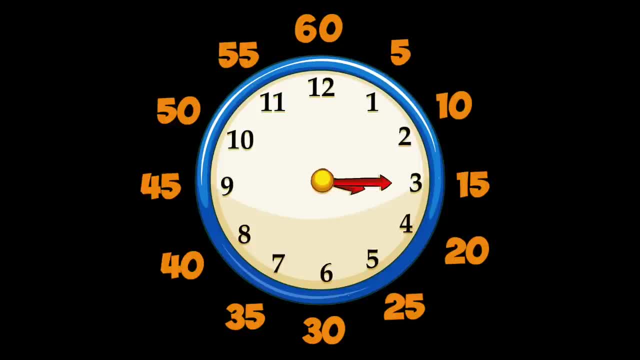 Notice how each number on the clock stands for one group of 5 minutes. So 3.15 is when the long hand is pointing to the 3 and the small hand has moved a little past the 3.. If we were to show 4.45, we'd start at 4 o'clock. 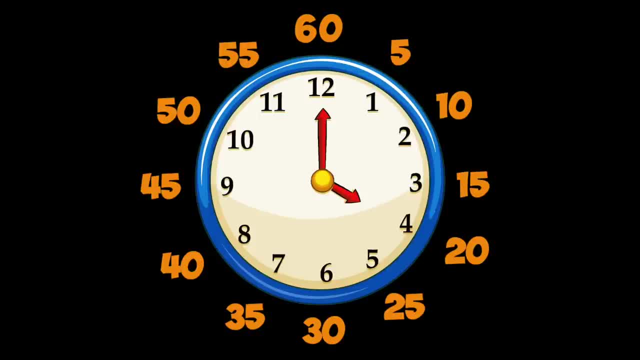 which is when the big hand's on 12 and the small on the 4, and then count by 5's until we get to 45.. 5, 5, 10,, 15,, 20.. 20,, 25,, 30,, 35,, 40,, 45.. 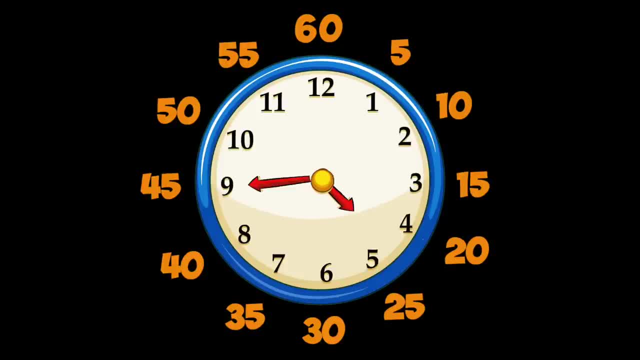 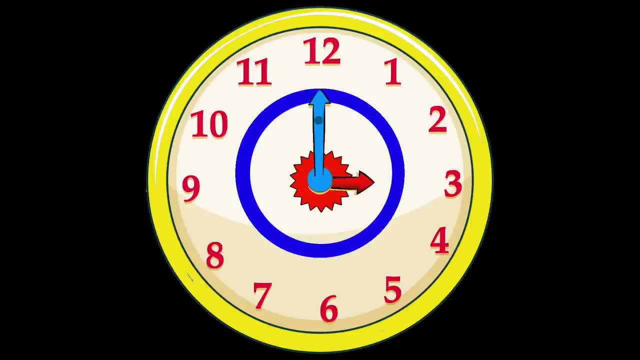 You can see that 45 is at the number 9 and that's 4.45.. Can you use a learning clock to make some of your favorite times of the day Have fun? And then came Thursday. Our class came in from recess and we had run around. 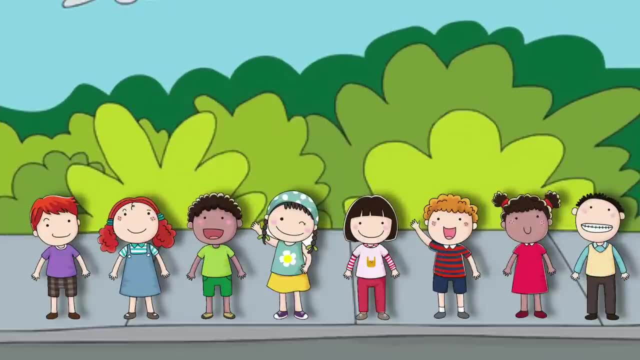 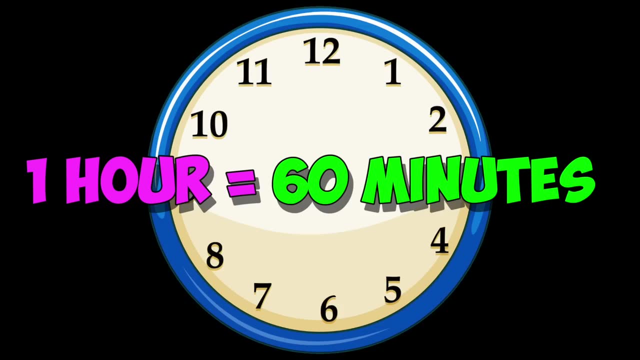 Now we were starving really bad. our tummies made this sound. Our teacher said there's chocolate. But we would have to wait Exactly for one hour. 60 minutes was our fate. Our teacher started singing a 60 minute song. 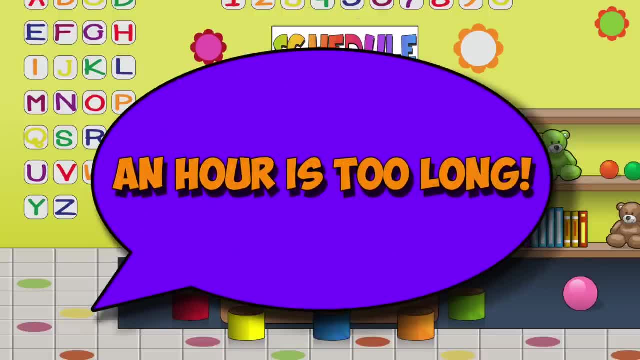 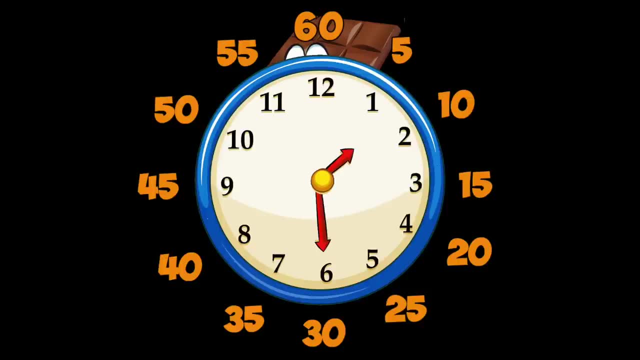 But every student wanted to sing. an hour is too long. It was 5, 10,, 15,, 20,, 25,, 30.. That's a half hour and we're still really hungry. 35,, 40,, 45,, 50,, 55,, 60.. 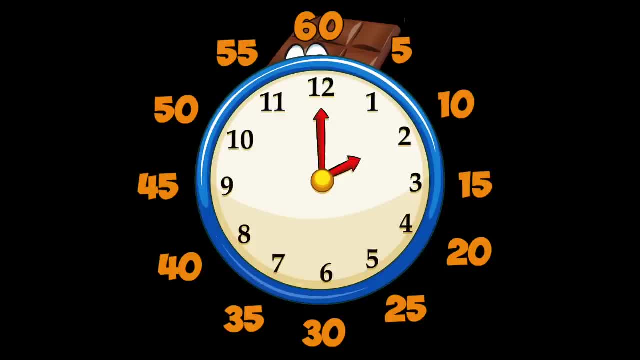 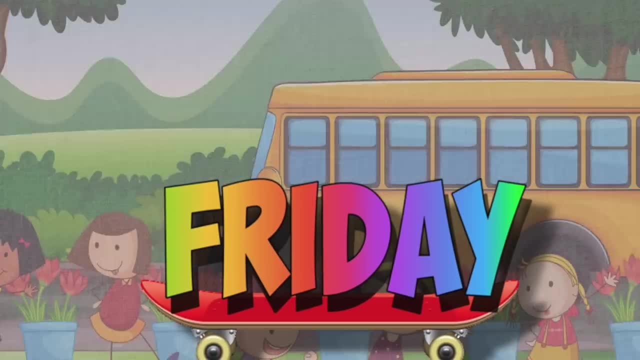 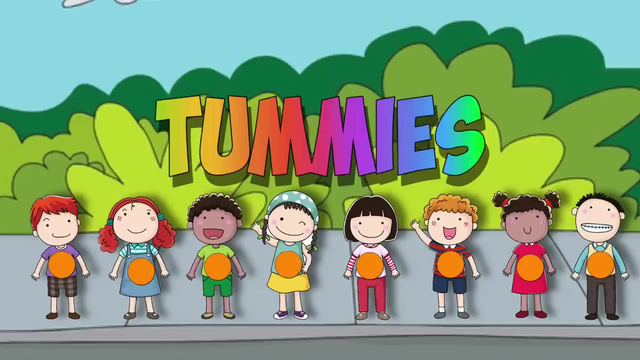 Where's our chocolate? Well, 60 minutes is one hour, So I guess it's chocolate time. And then came Friday. Our class came in from recess and we had run around. Now we were starving really bad. our tummies made this sound. 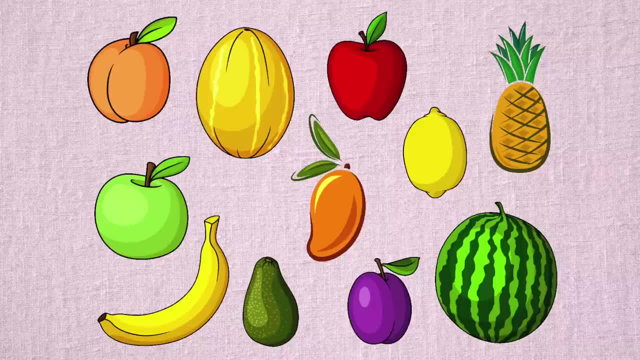 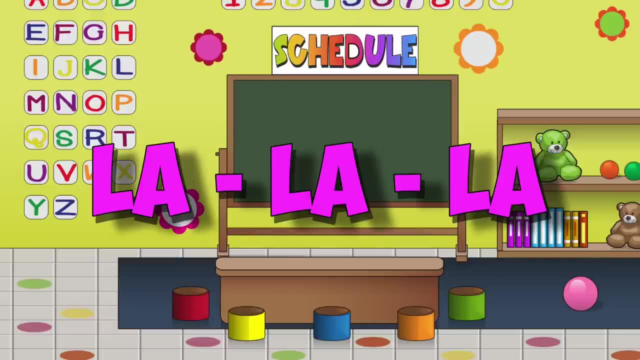 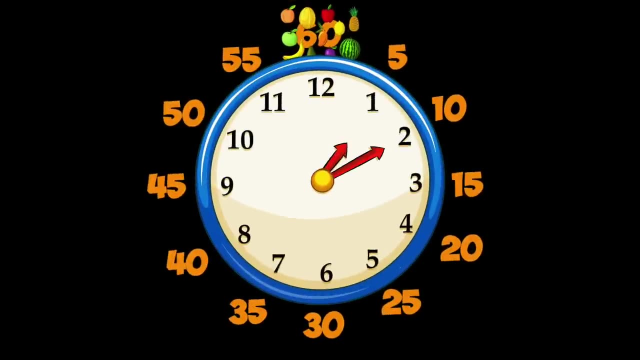 Our teacher said there's fresh fruit, But we would have to wait Exactly for one hour. 60 minutes was our fate. Our teacher started singing a 60 minute song, But every student wanted to sing. an hour is too long. It was 5,, 10,, 15,, 20,, 25,, 30.. 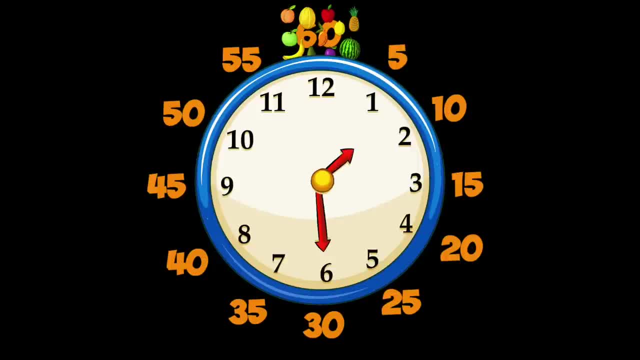 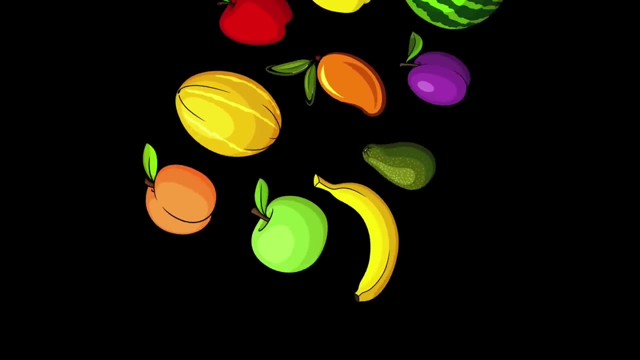 That's a half hour and we're still really hungry. 35,, 40,, 45,, 50,, 55,, 60.. Where's our fresh fruit? Well, 60 minutes is one hour, So I guess it's fresh fruit time. 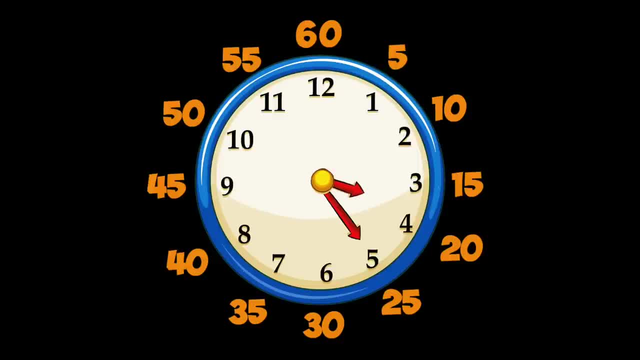 It was 5,, 10,, 15,, 20,, 25,, 30.. But every student wanted to sing. an hour is too long. It was 5,, 10,, 15,, 20,, 25,, 30.. 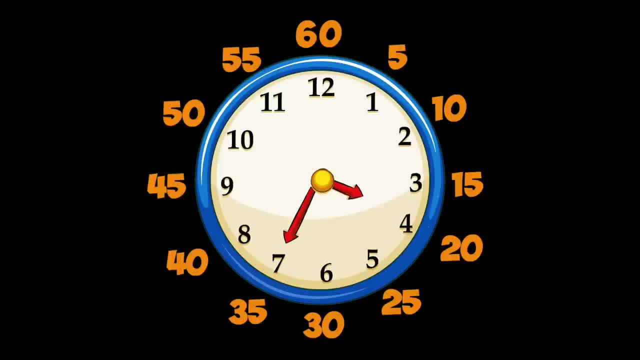 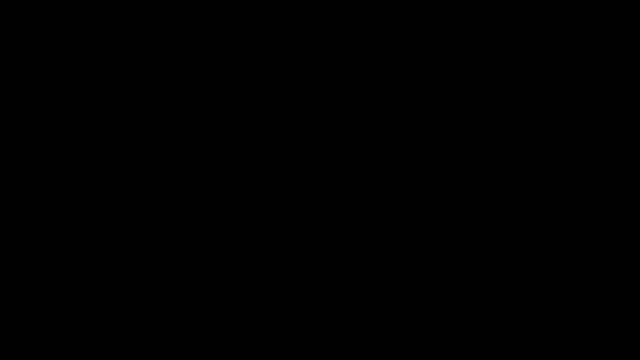 That's a half hour and we're still really hungry. 35,, 40,, 45,, 50,, 55,, 60. That's one hour, So I guess it's fresh fruit. He saw a seed. It was a big way and a seed. Alright, There it is. It did come back from a tree, A new tree, Little fixed pediatric tilapia. Well, that was really tough for him because we're talking a lot about bio- These are soil Materials- But it's really really good ever since. 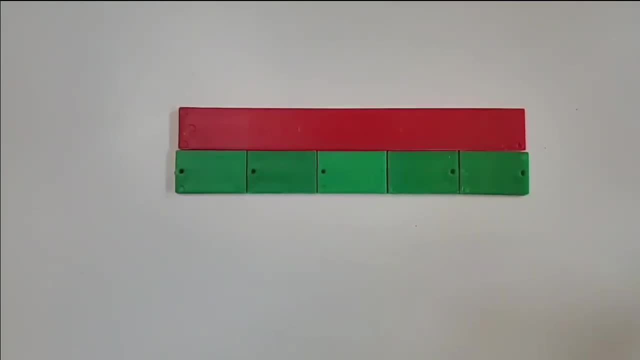 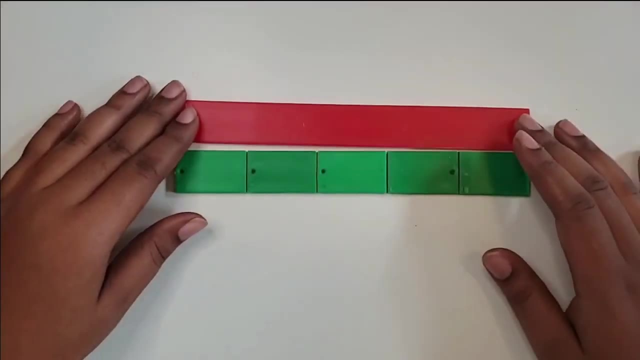 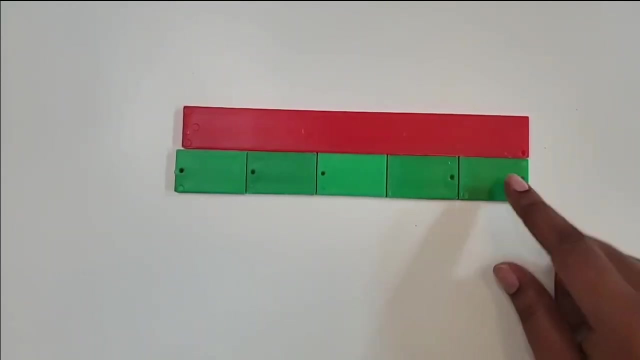 In this video, I'm going to share with you how to subtract fractions with the same denominator using fraction bars. Here we have our whole and we have some fractions. It takes one, two, three, four, five of these fraction bars or tiles to make up the whole. So, since it's five of them, 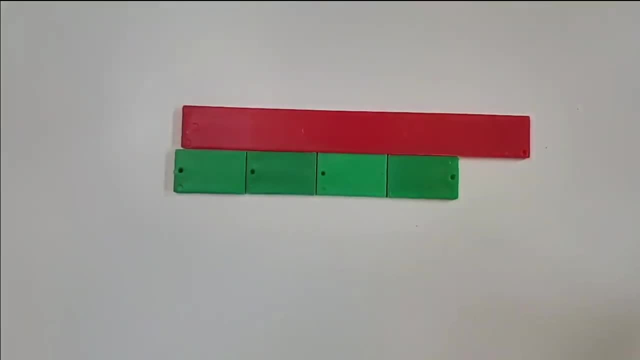 these are fifths. Well, what if I wanted to use four fifths and take away two fifths? So I have four fifths here. I'm going to take one fifth, two fifths away. Now how many are remaining?